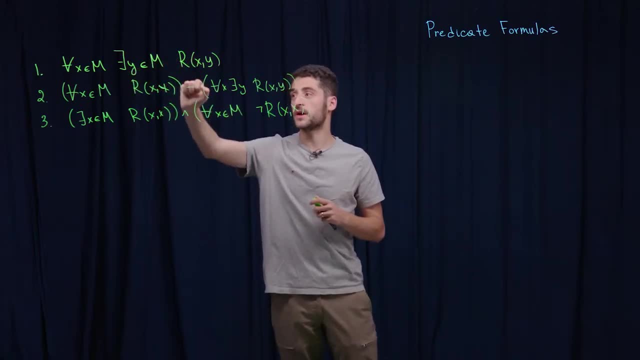 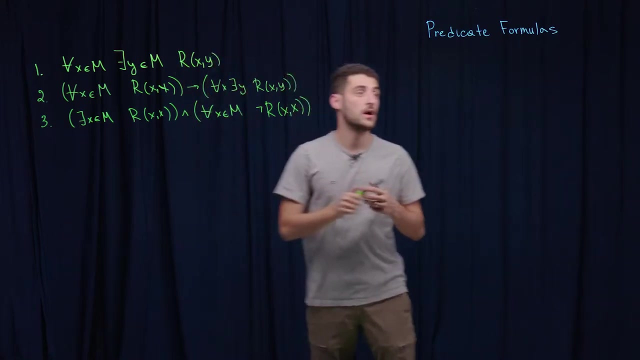 the first formula and note that we have two undefined symbols here. We don't know what it means M and what it means R. Obviously, M should be a set and R should be a relation and, depending how we define these two objects, this formula may be a true or false. For example, if M is a set of 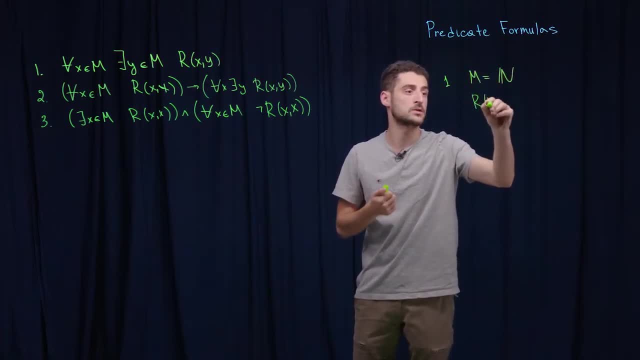 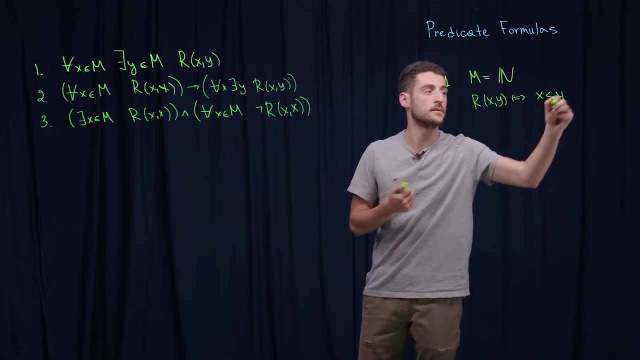 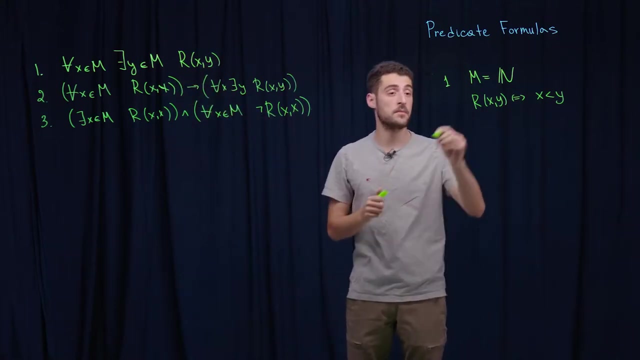 positive integers and R of XY is X is less than Y. this formula is obviously true because for every element there is a bigger element. But if M is still the set of positive integers, but r, where X is 0, will mean that R is less than N. 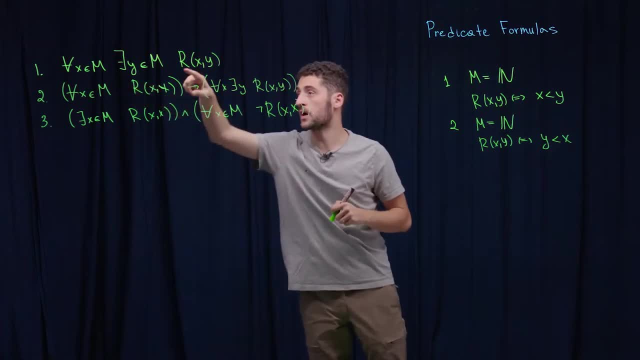 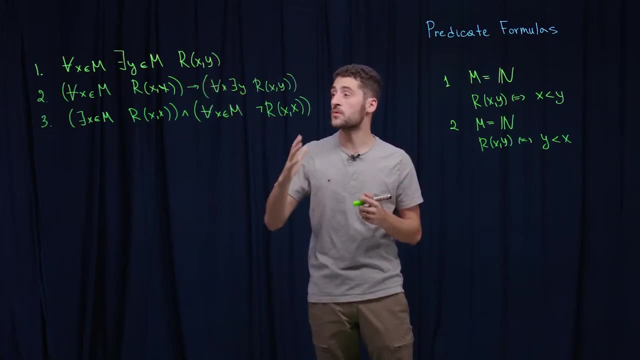 and that is smaller than X. But if M is a good set of positive integers, it will still be the set of positive integers. So M is equal to a set of positive integers. The second formula is true Whenever we define M and R and when we define a set of positive. integers. this formula is obviously true, But if M and R are again separate. So for each set of positive integers, each set of positive integers plus Y is equal to 1.. If manyverständそれは shrug. coordinated statement 159 00 delegation. 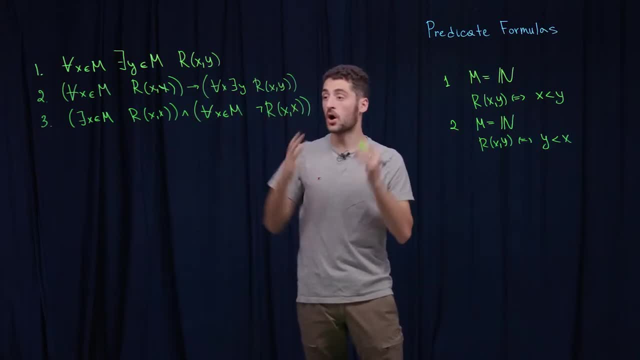 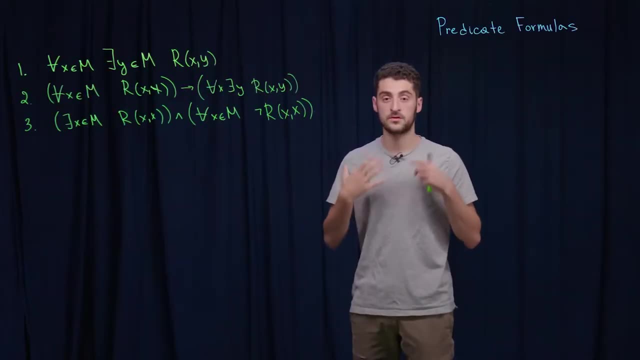 x bulleted downется 0 because the y criteria is the set of positive. the third formula is always false because this is the negation of this. so they together gives you a contradiction. in other words, in order to define predicate formulas, we need to define what kind. 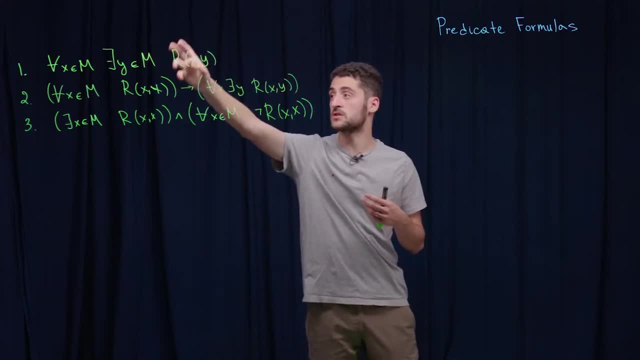 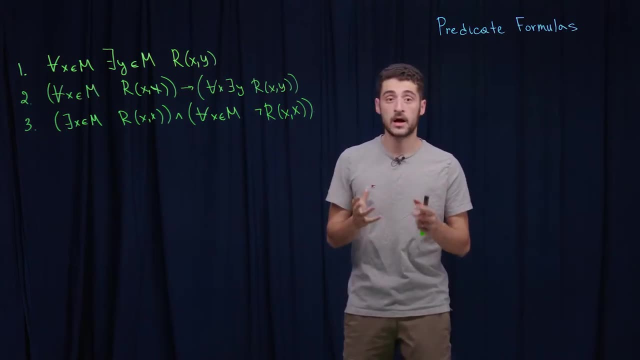 of symbols we can use inside, what kind of symbol for relations, symbol for sets or functions, and we also need to define what these symbols mean and in the predicate logic we separate this to definition. the definition of a set of symbols we use is called the signature and the definition of what. 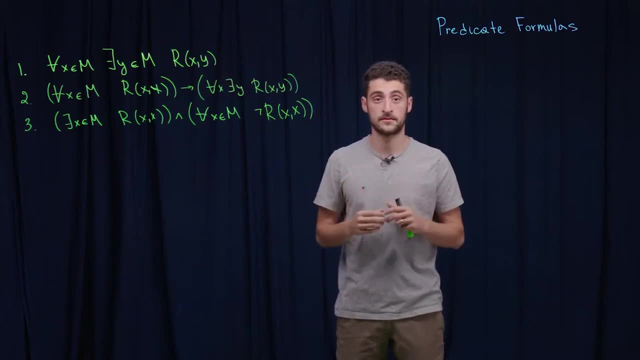 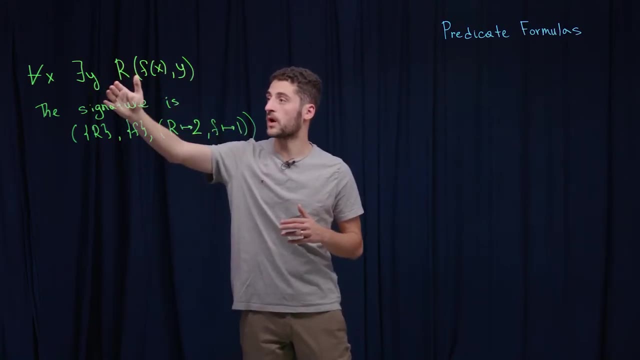 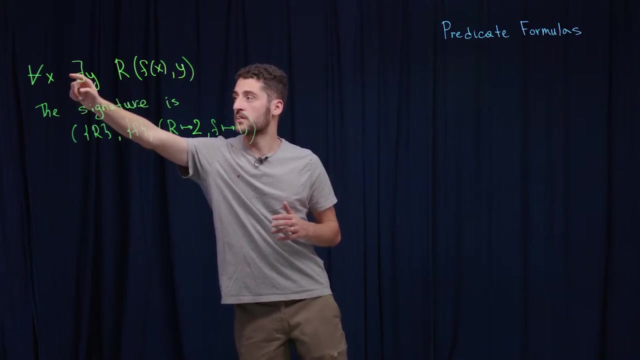 they mean is called structure. first we need to define signature. so consider this formula. it says that for all x exists y, such that r of f of X, Y is true. note that we dropped that x belongs to M and y belongs to M, because we'll assume that all the quantifiers are equal, so complimenting. 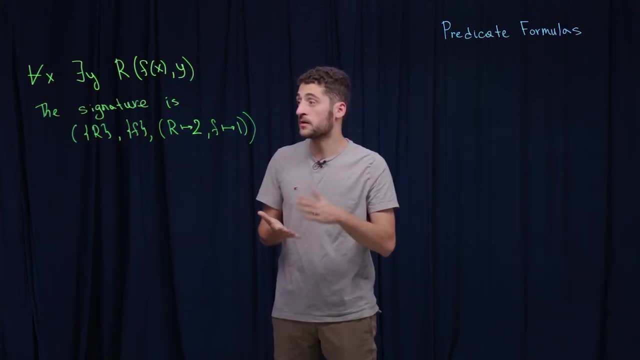 X. so instead of the letters that are x, fl, sy, fl or r or f. so if we think about it simply, if we have most symbols, we produce significant Googling behavior, Plus that we have the are over some fixed set which will be defined in the structure. So right now we 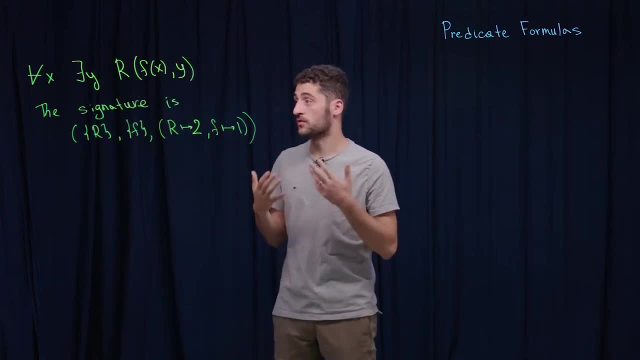 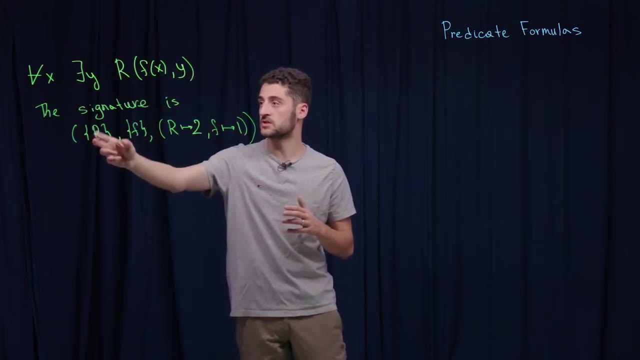 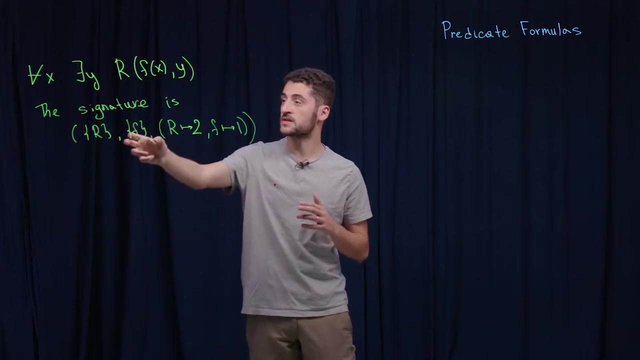 write all the formulas with quantifiers without the restriction over this of the set. And in order to define the signature of this formula, we need to define the set of all the relation symbols, the symbols for relations. In this case, there is only one symbol for the relation, it's R. We need to define the set of all. 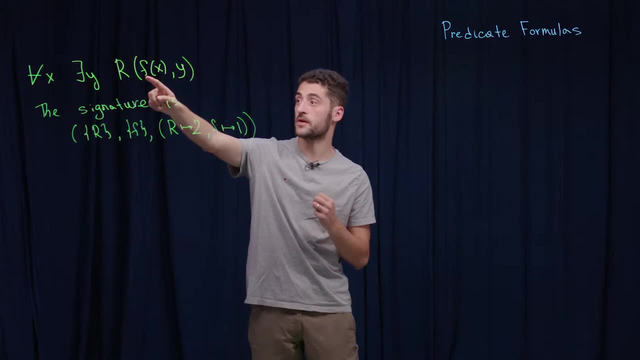 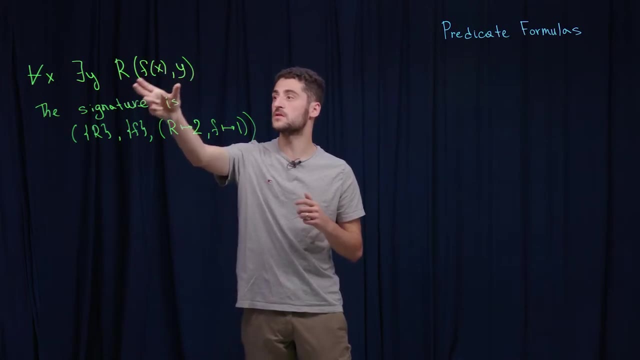 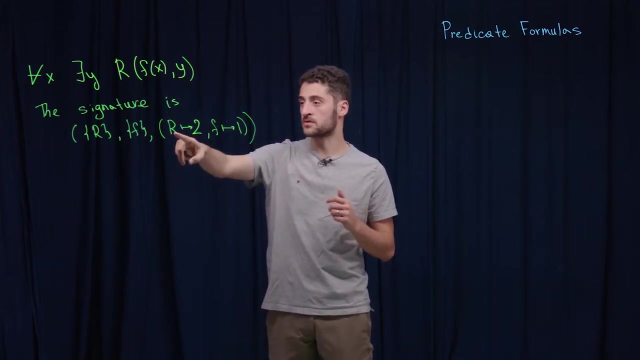 symbols for functions. In this case we have only one symbol for the function, F, And we also need to say how many arguments this relations and function takes. For example, R can take two arguments, so the third parameter of the signature says that R has two parameters and F has only one parameter. 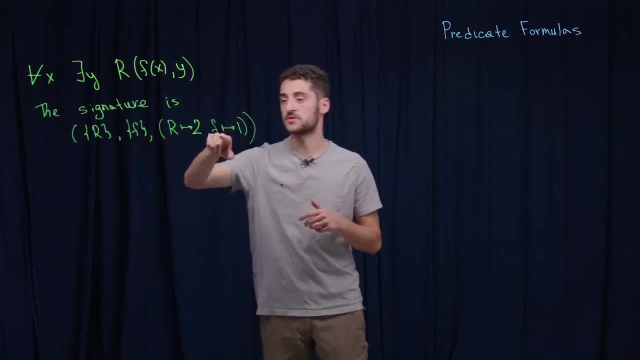 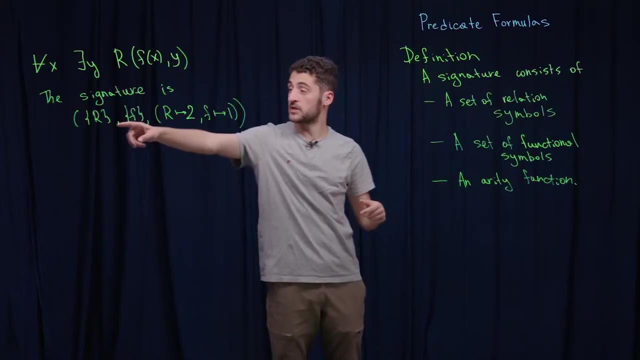 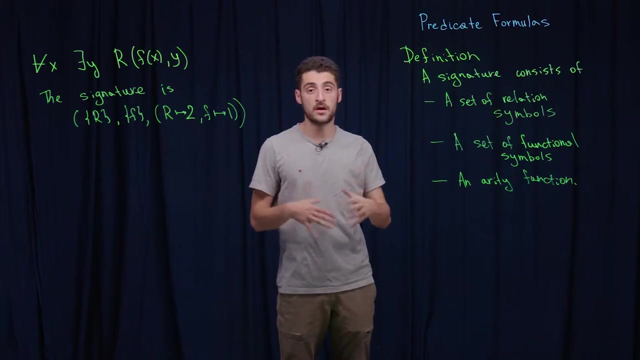 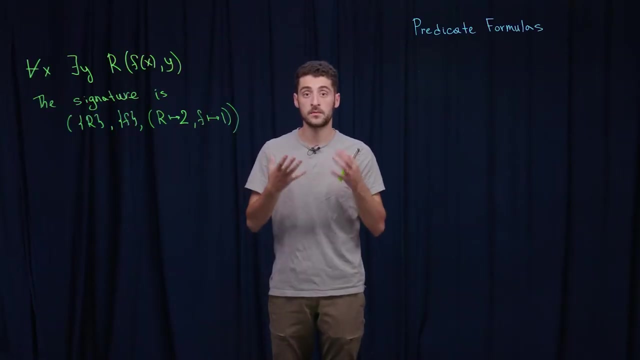 so the third part of the signature says that F has one parameter. In other words, signature consists of three elements: a set of relations symbols, a set of functional symbols and finally, an arity function saying that what are the arities of relations and functions we can use? Now we may define predicate. 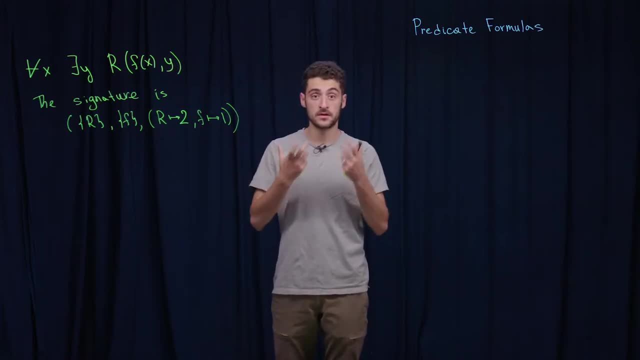 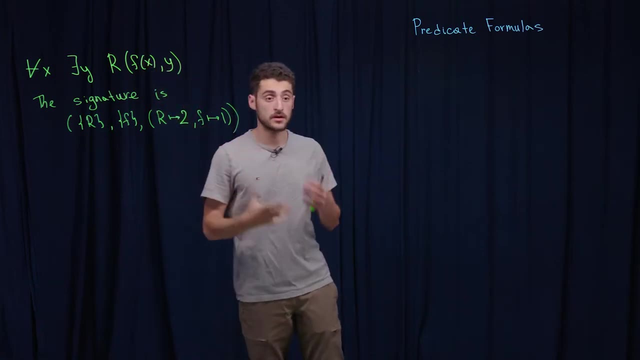 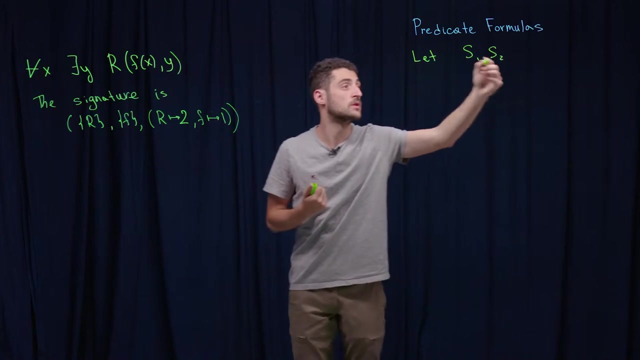 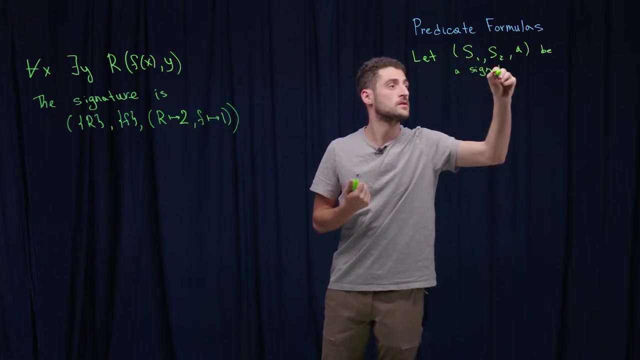 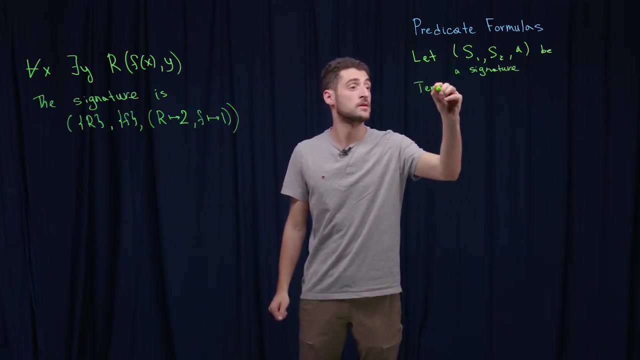 formulas. First we need to define is the notion of a term. For example, in this formula, f is a term and y is a term. Let's do this, So let S1, S2 a be a signature, For example. it's something like this: Then term is either: 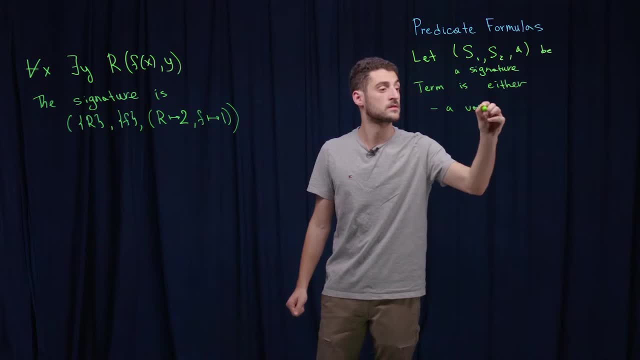 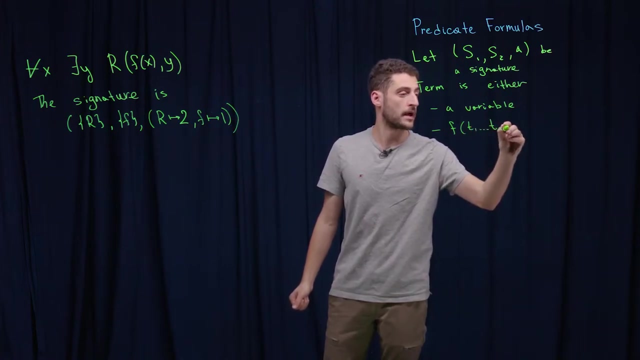 a, a, a, a, a variable. For example, y here is a term and x here is a term, Or it's f of t1, ta-ta-ta ta of f, where t1, ta-ta-ta ta of f are. 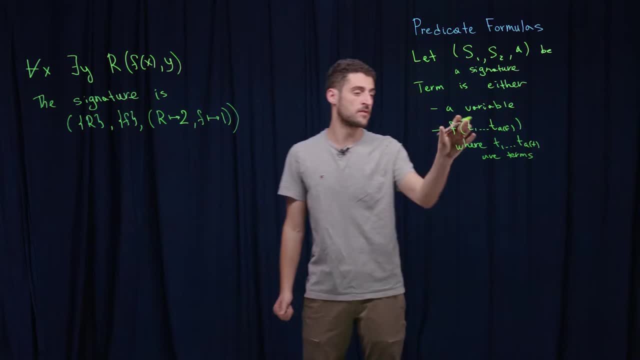 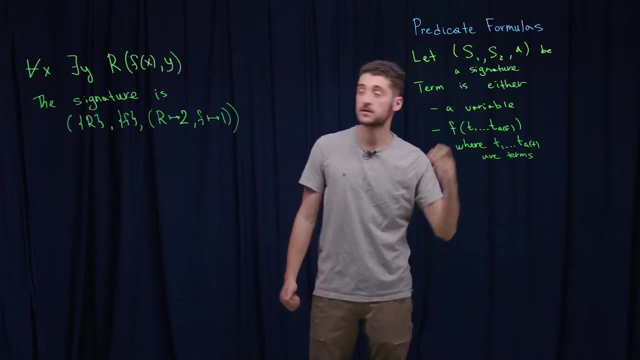 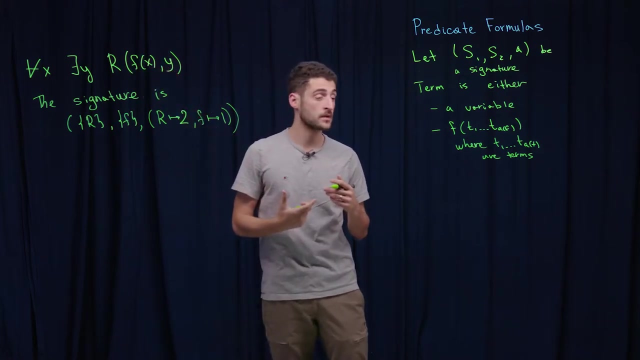 terms. So you should remember that the function should take a of f arguments. so we need at least a of f terms. And for example, here f has one argument and x is a term, so f of x is also a term. And finally, when we define terms, we can define formulas. 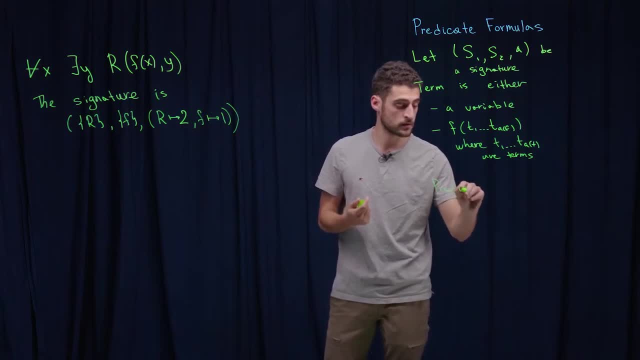 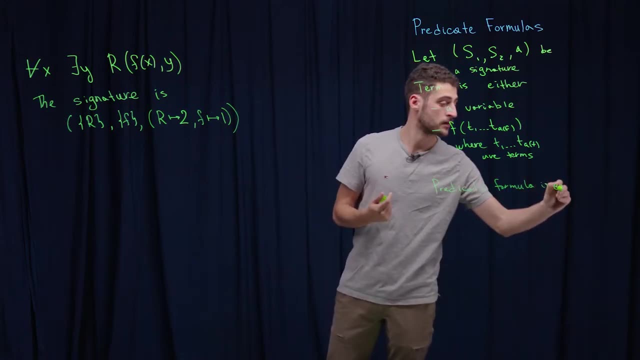 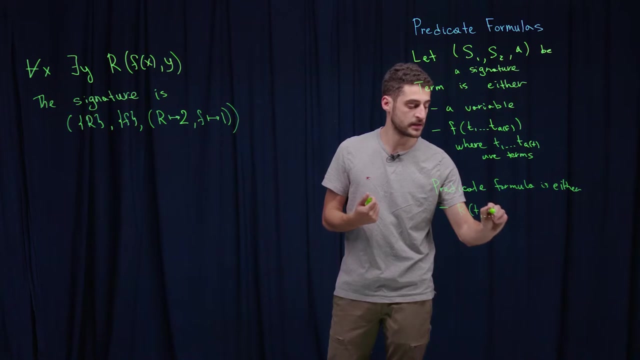 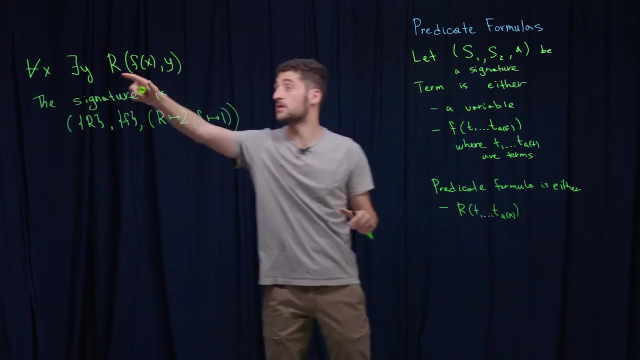 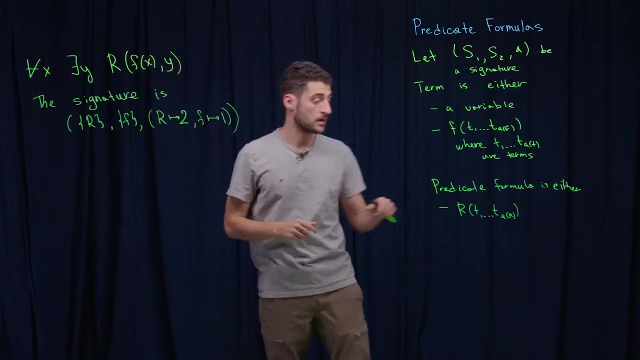 So predicate formula is either r of t1, ta-ta-ta, ta of r, So it's a relation of some terms. For example here: this is a formula because it's a relation of one term and another one, Or it can be negation. 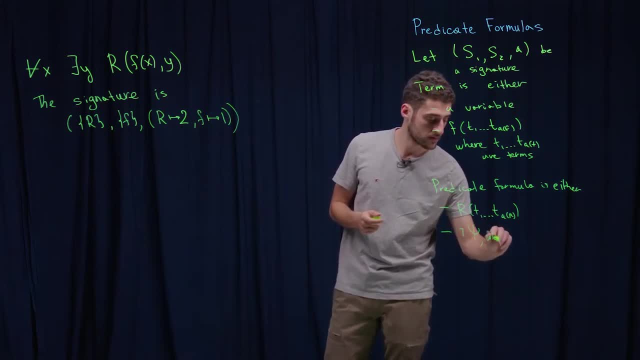 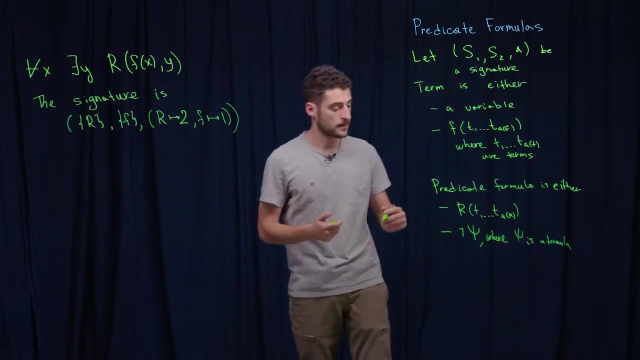 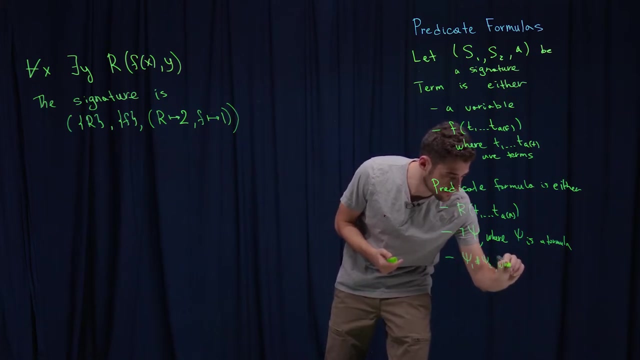 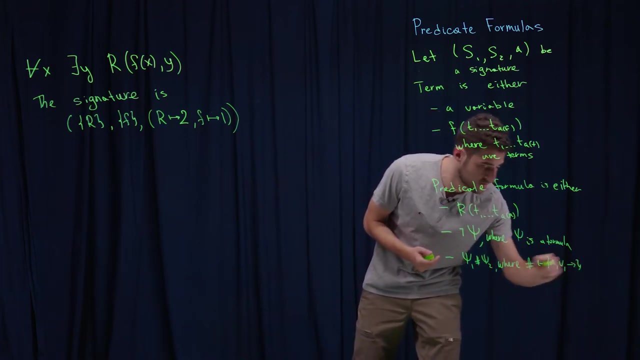 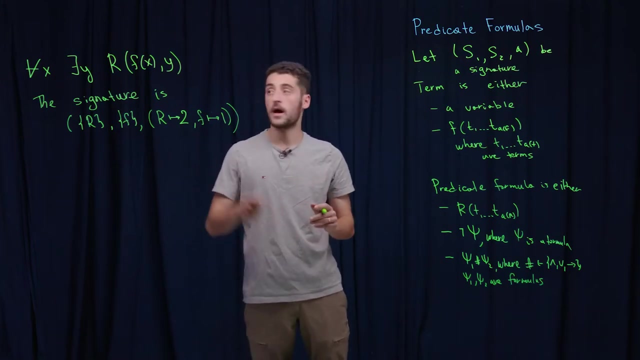 of psi, where psi is a formula. It can be also psi 1, sharp, psi 2,, where psi sharp is, and or or implication, And psi 1, psi 2 are formulas And finally it's. it can be also a predicate and a formula. 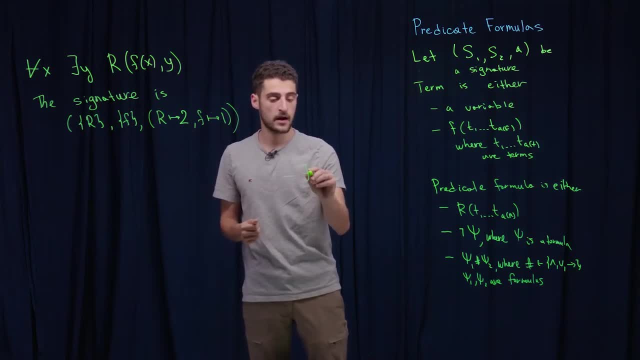 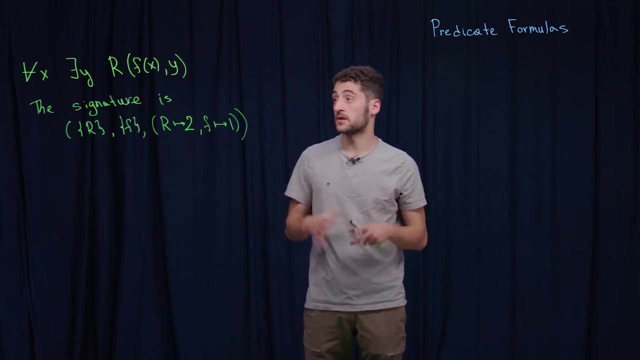 So it can be. exists x psi of x. Psi of x means that the formula depends on x, Or it can be for all x psi of x. Now we are ready to define the formula. We are going to define the structure, in other words, how to interpret the formula. 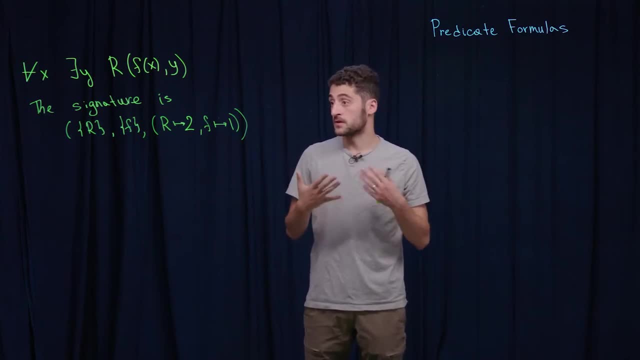 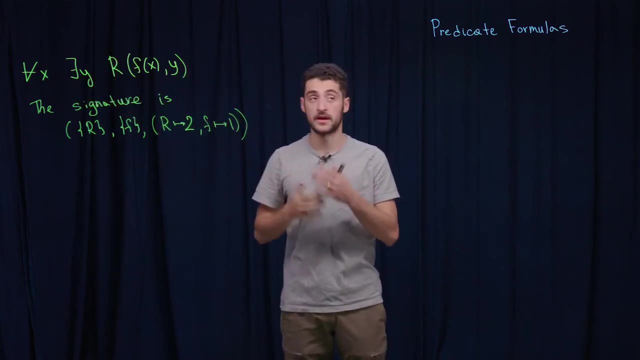 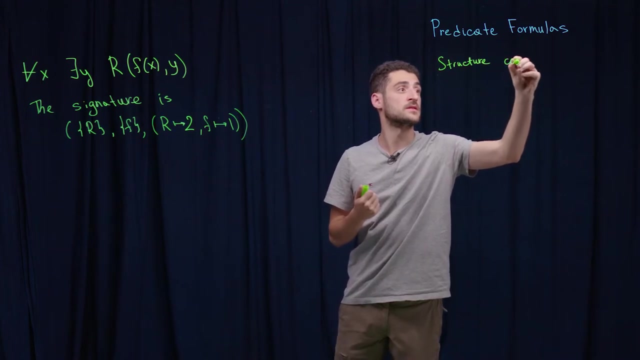 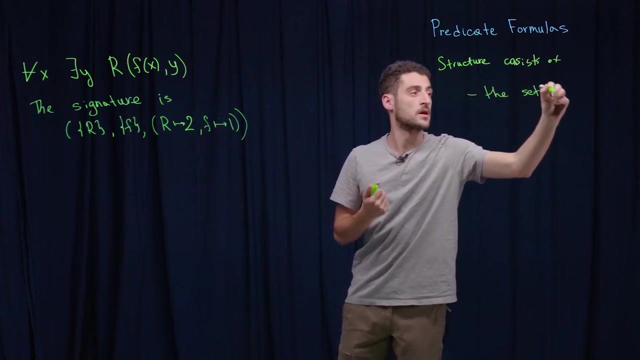 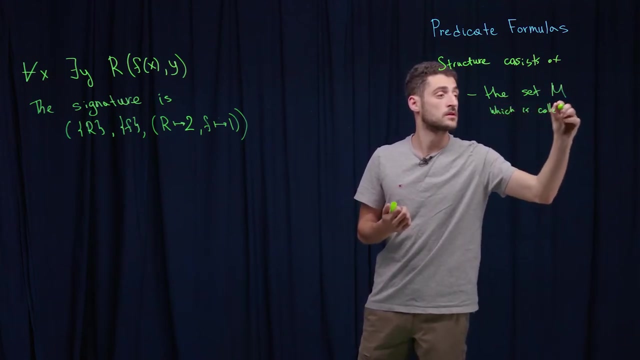 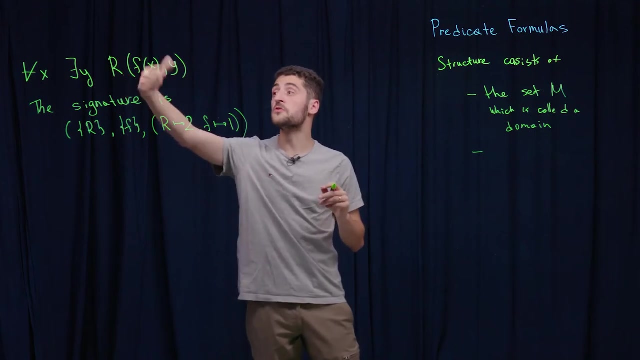 how to compute the value of it. First part of this is the set M, which is saying over which set all the quantifiers are taken. So structure consists of the set M, which is called domain. It's also needs to give an interpretation to every relation symbol.